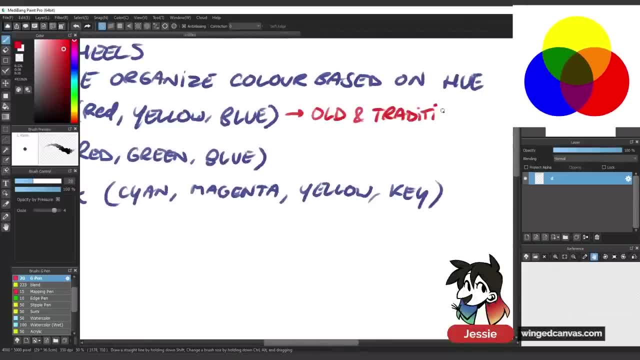 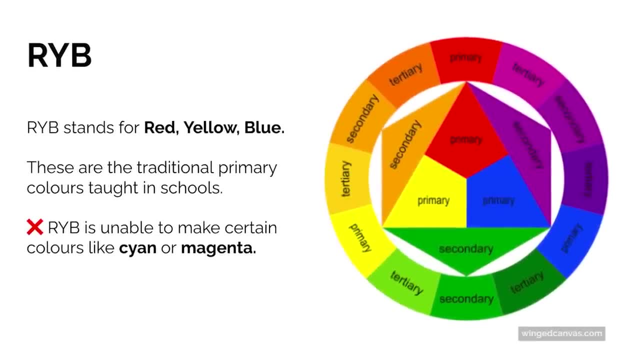 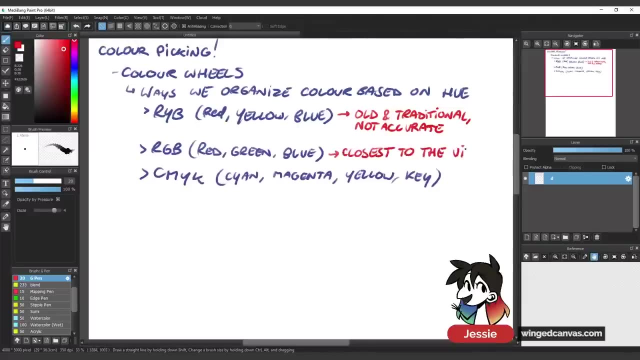 of black RYB. we will be using RYB today just because it's considered the beginner's color wheel. It technically is not 100% correct, but it is like an old and traditional way of thinking about it, Right? don't tell your teachers. So RGB is our most accurate color wheel, which means that 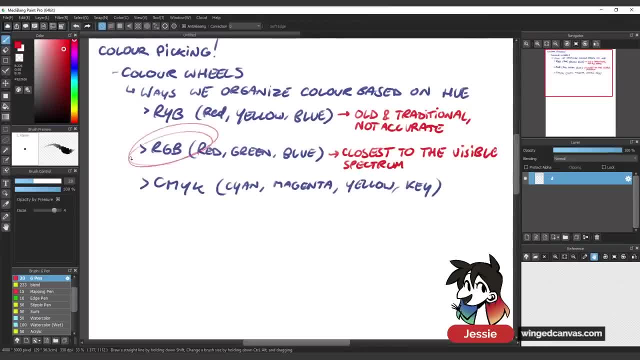 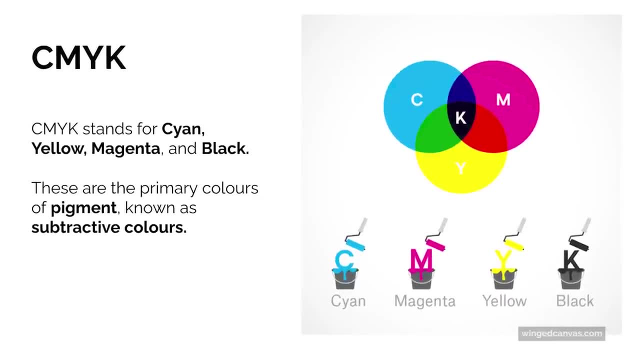 red, green and blue are our primary colors, So RYB is our most accurate color wheel, Right? so RGB is the closest to the visible spectrum that we've gotten. And then CMYK is a printer's colors, right? So if you go to print something, right, that's what you use. CMYK tends 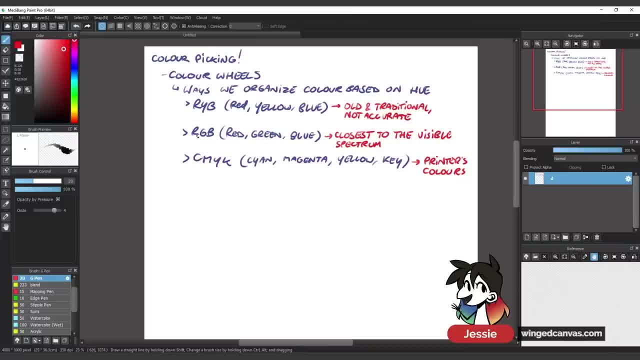 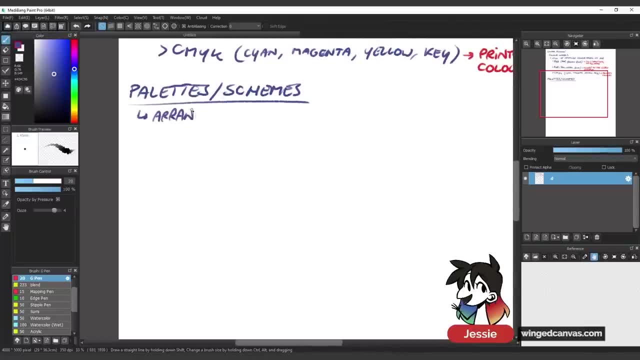 to be a little more dull, but it does have a wider range of hues compared to RYB. So color palettes and schemes are arrangements of color to have different effects and moods. right, When you have a color palette they usually give off. different moods they usually give off. 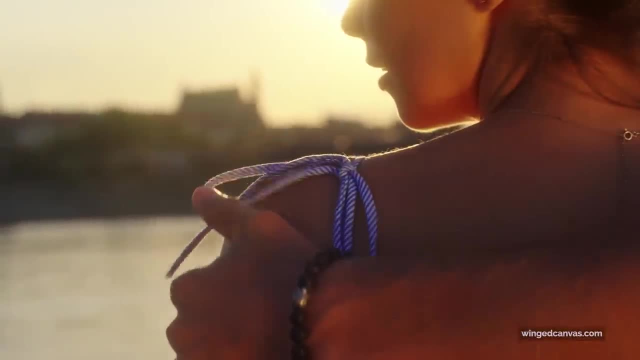 different moods and they usually give off different moods. So if you have a color palette, you usually use them in different situations. So our palettes and schemes are just putting names to those moods and how you can use them. Let's start off with analogous. This is the one that 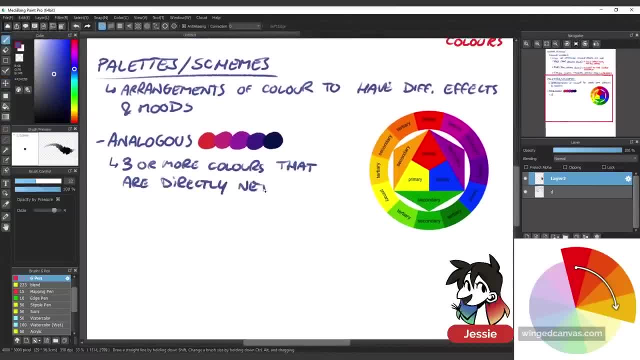 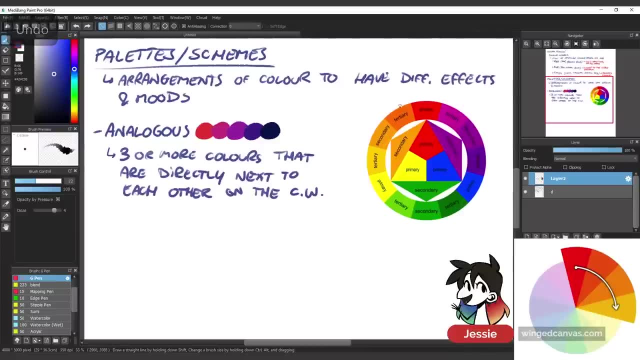 most people like to use. Analogous color schemes are three or more colors that are directly next to each other on the color wheel. So if I go from red all the way down to blue, down here, that's an analogous color scheme, right. I could go in the opposite direction If I went from red. 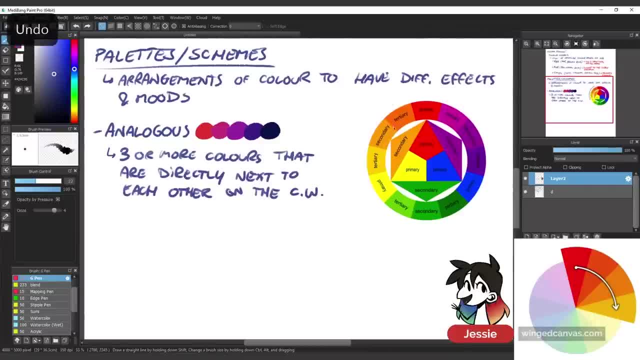 orange down to yellow. that's also analogous, right? It's just colors that are directly next to each other on the color wheel. This is a palette that you can't mess up. It's a very, very open-ended palette. It's a very, very open-ended palette. It's a very, very open-ended. 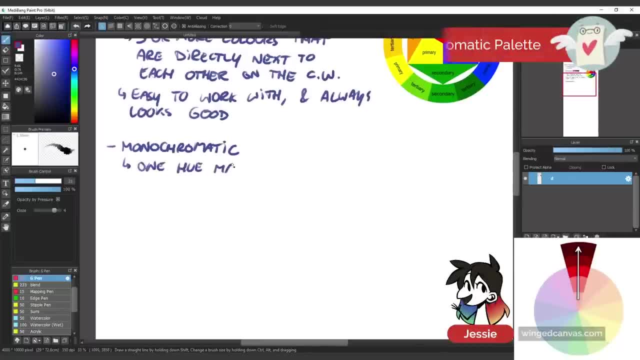 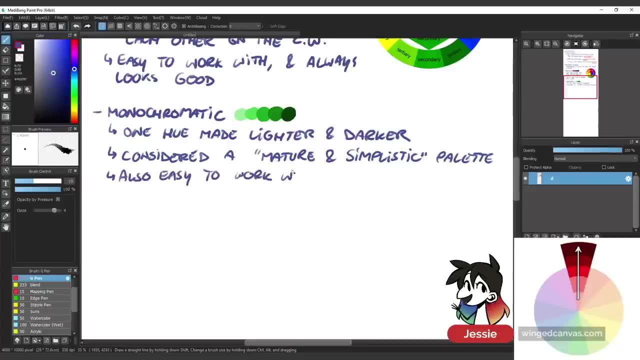 palette, but at the same time it can get very, very boring. So monochromatic schemes are one hue made lighter and darker. right. It's considered a mature and simplistic palette and it's also easy to work with. but a good grasp on values is needed. If you're not very good with your values. 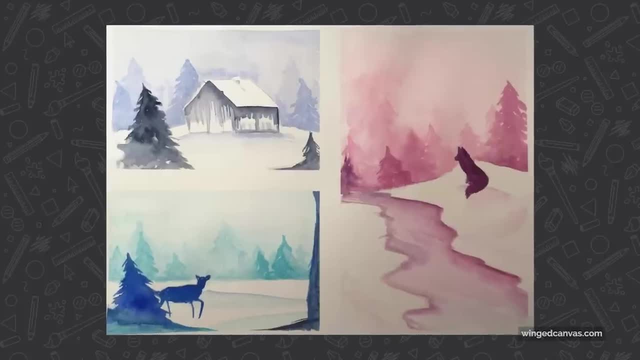 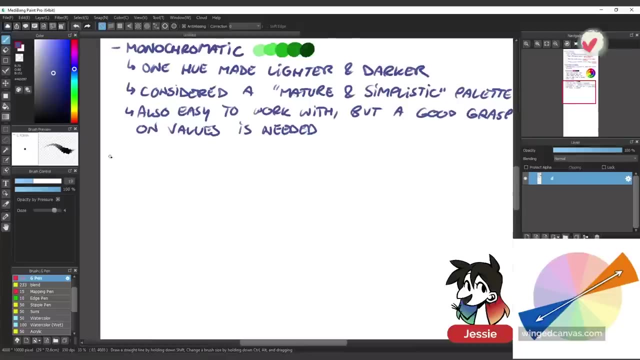 you will not be able to do monochromatic very well, And that's because with monochromatic color schemes- right, you don't have color to rely on to distinguish forms, You just have your values and your saturation. So complementary palettes colors directly across from one another on the 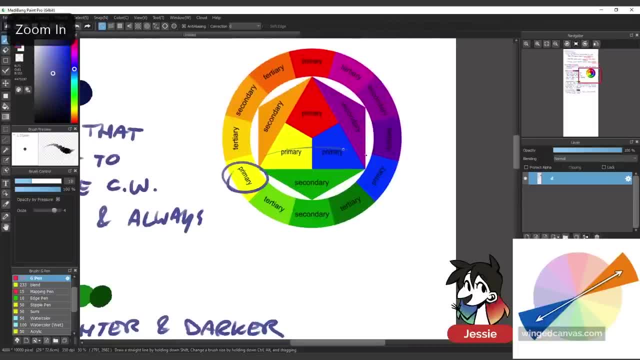 color wheel. The thing is that with RGB it's yellow and blue that are directly across from each other, but on RYB it's yellow and purple. It's two colors that are directly across from each other on the color wheel right. So with 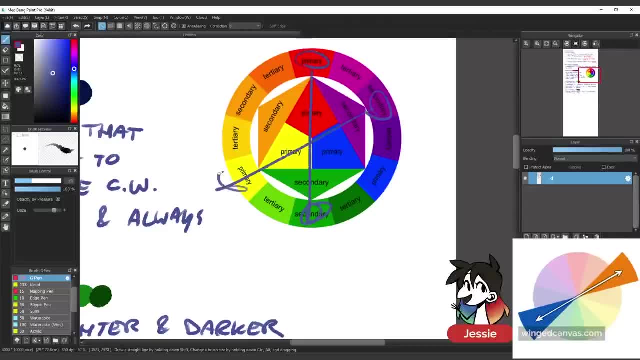 RYB. red and green are complementary, purple and yellow are complementary, orange and blue are complementary. You could also be working with tertiaries. So if you had yellow-green which is directly across from red-purple, right, that's also considered complementary. So the traditional 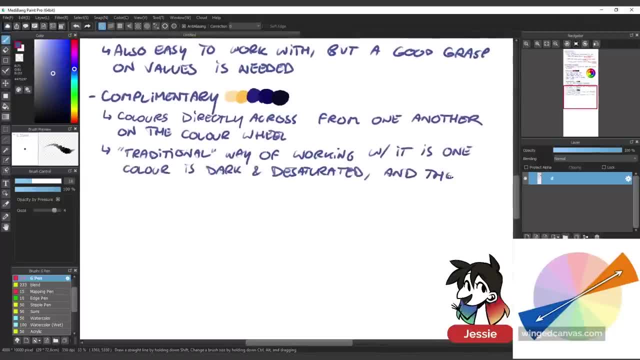 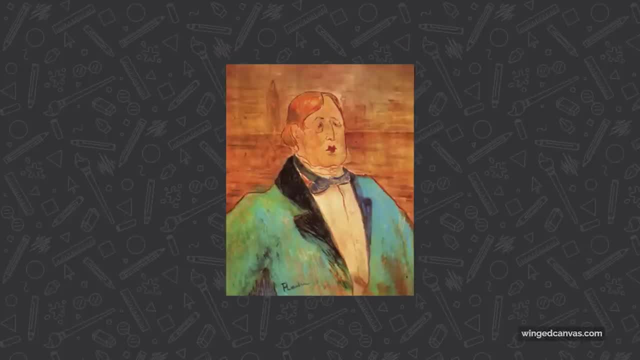 way of working with it is what one color is dark and desaturated, the other is bright and saturated. So complementary colors can be a bit trickier to work with, because sometimes you just might not get a good looking color combination and then it'll end up looking like a Christmas tree. 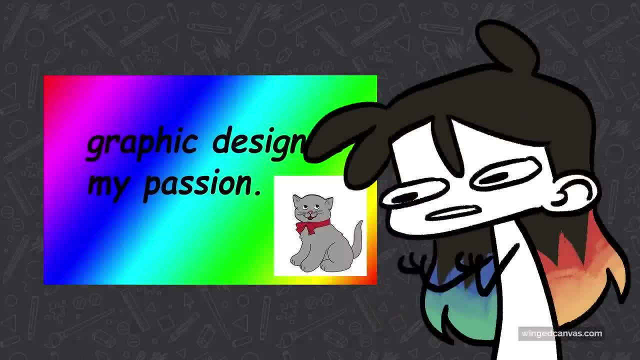 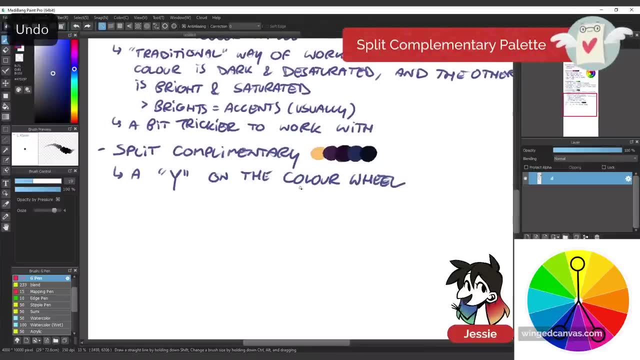 or it just looks ugly, right. Sometimes it just looks like a graphic design is my passion kind of poster which is like: not what you want, obviously. So split complementaries, create a Y on the color wheel. So when I say Y, it starts at one color and then branches off in two different ways, like that. 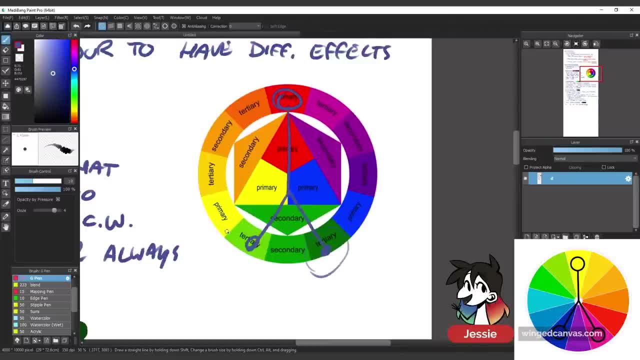 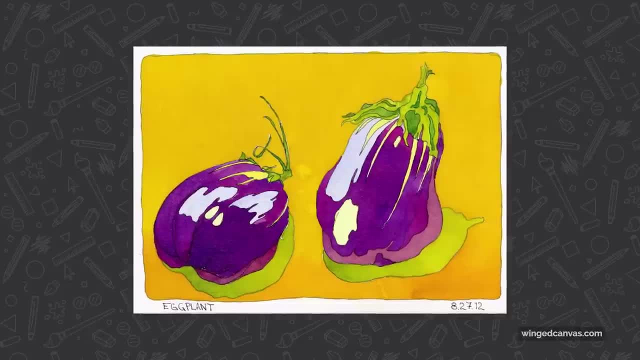 right. So if I start with the primary of red, then I'll end up at blue-green and yellow-green. It's a more thorough complementary, But complementaries can be very, very tricky to use. Usually you need a good idea of balance and how to use it. And then one last one, which is triadic. 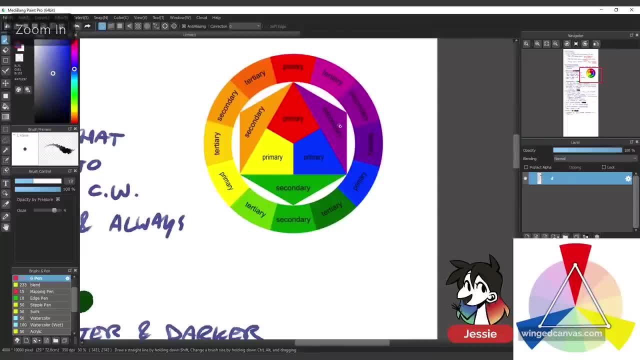 So triadic colors will create an equilateral triangle on the color wheel. So when you create an equilateral triangle on the color wheel, right? so if we start at one primary, then we'll touch the other primaries as well. So if I start at red, then I'll also be picking yellow and blue. 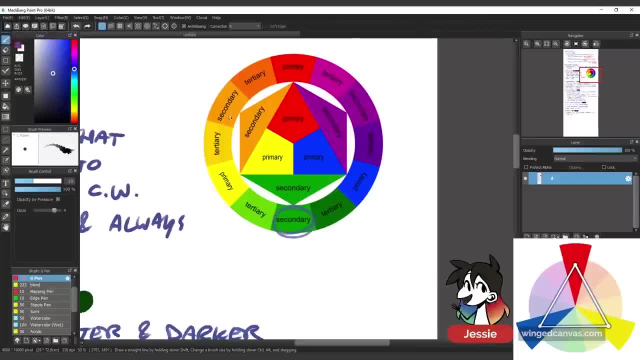 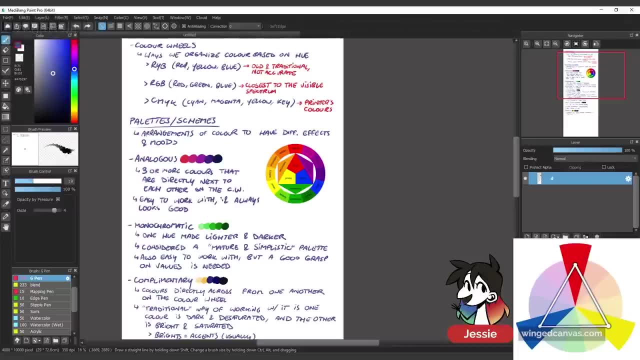 On the contrary, if I were to pick green, then I would also pick orange and purple, So that also creates an equilateral triangle. So just as long as you have all those colors equidistant to one another, then you have a triadic color scheme. Triadic color schemes- you see a lot. 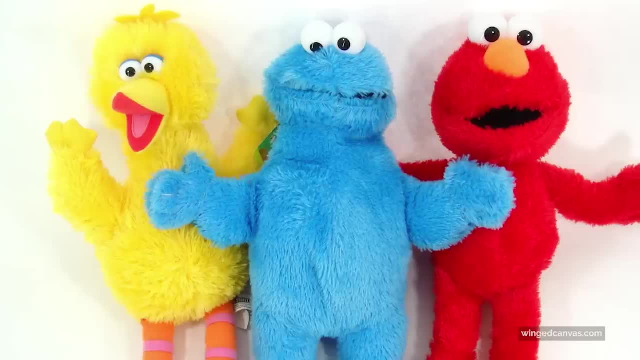 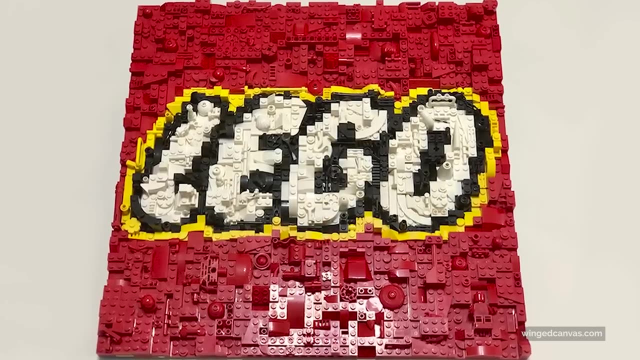 within children's products, children's products, children's games, or like children's toys, Lego, even. look at the logo right, The colors that you see most often. they're usually very bright and triadic. That's because triadic color schemes are just the brightest. They're very, very lively. 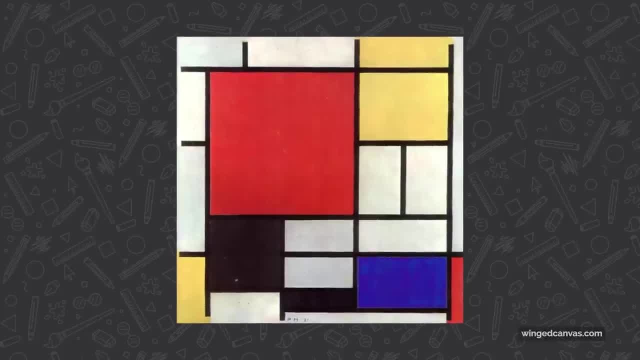 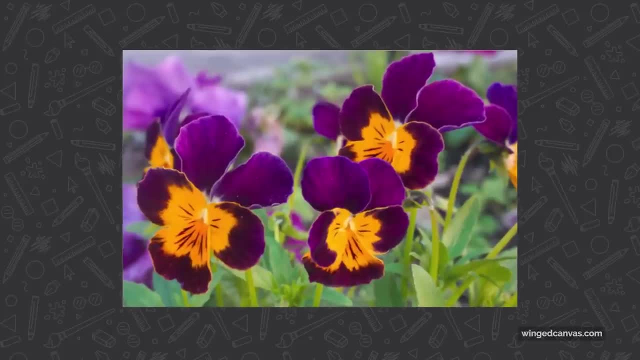 And triadics are very difficult to work with. It's one that can be pretty tricky to work with if you're not very familiar with color. So triadic is usually not one that people start with. but once you get a hang of the color and whatnot, triadic becomes a favorite of a lot of people. 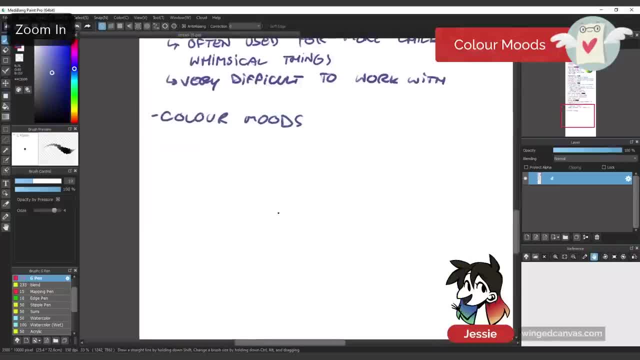 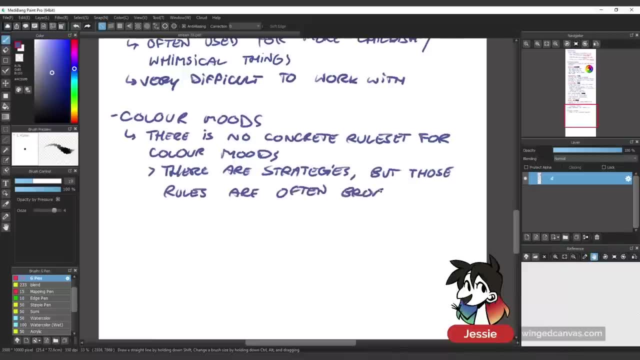 Let's talk about color moods, because this is how you actually pick your colors. There is no concrete rule set for color moods, unfortunately. right, Can I teach you about them? Absolutely. But even then, you're going to have to take what I say with a grain of salt, because there are strategies to 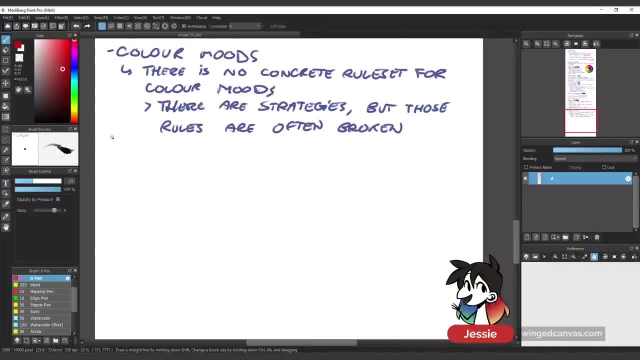 work with color in order to create certain moods, but those rules are often broken. So let's talk about HSV, which is color, is hue, saturation, value, So let's start with value. A lot of the times when people add lighter, 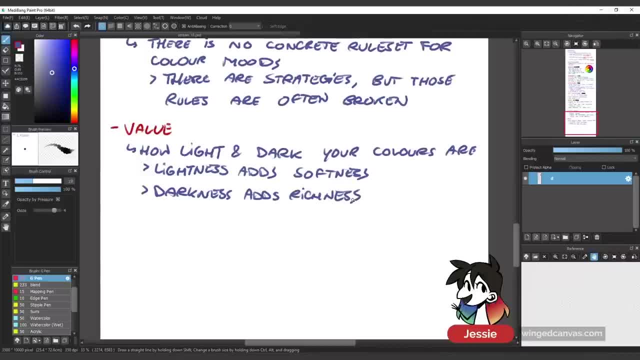 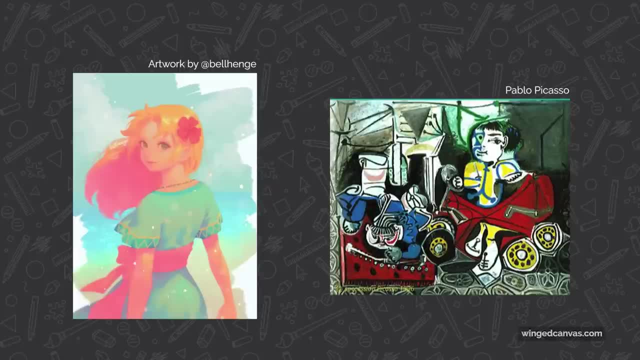 colors: nice pastels, light, fluffy colors, right, Those tend to be a lot softer, They're a little bit easier on the eyes. But your darkness, darker colors add a richness, They add a bit more of a mysterious value. They give it a bit more of a sharper look, I guess. But you need your lightness. 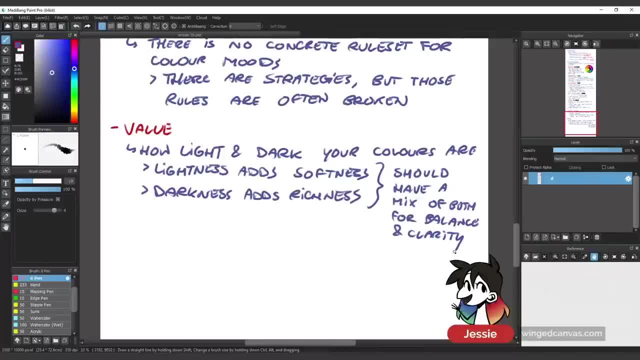 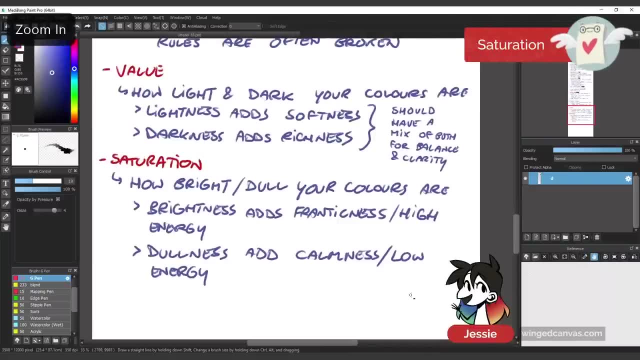 and your darkness with your values. in order to create a balanced looking piece, You should have a mix of both your lightness and darkness in order to have balance and clarity Saturation. It's easy to say: bright equals positive and dull equals negative. That's a very common one. 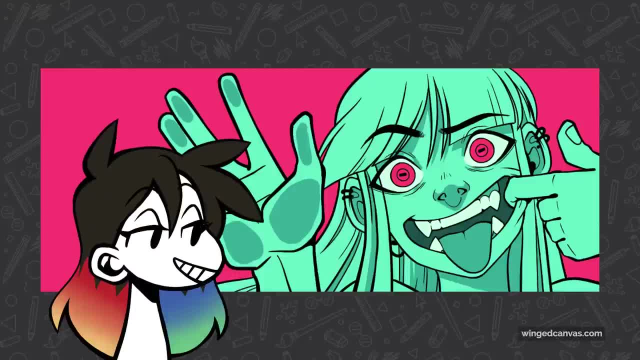 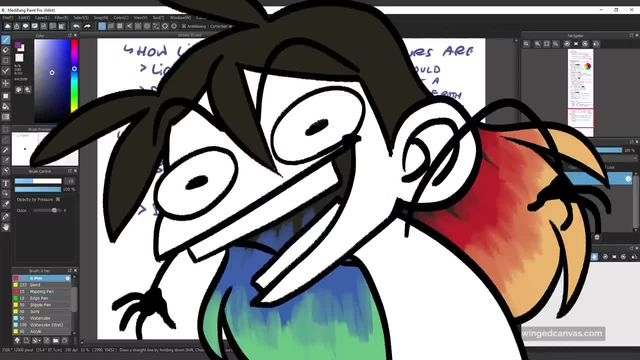 but not necessarily true. A lot of eye strain pieces are very, very negative. They tend to be a bit darker in terms of their subject matter, but they're still incredibly bright, which means that it adds a sense of franticness to it. Panic is still a very high energy emotion. It's not a 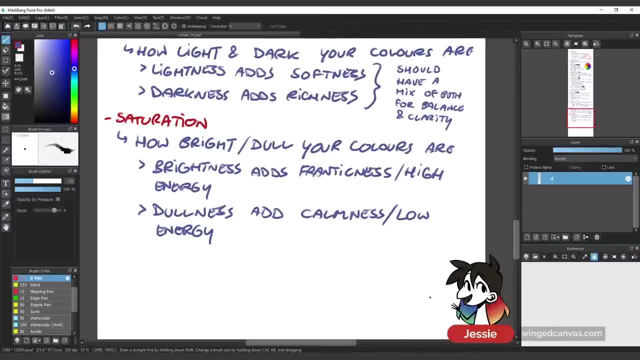 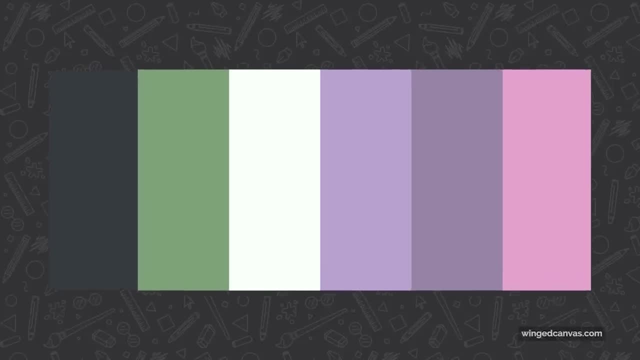 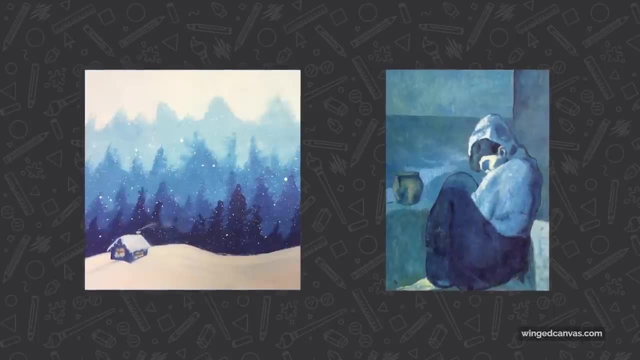 yeah, So a lot of desaturated stuff. The energy could be positive, It could be negative. A very calming, relaxing piece could be used with a lot of light, dull blues. That blue gives it a nice calming feeling, depending on the value added to it. Or it could be a negative thing, right, Maybe? 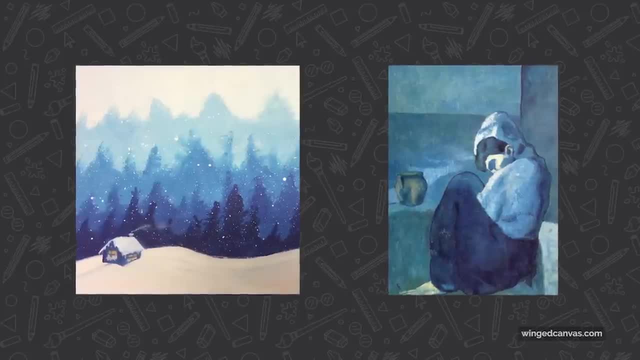 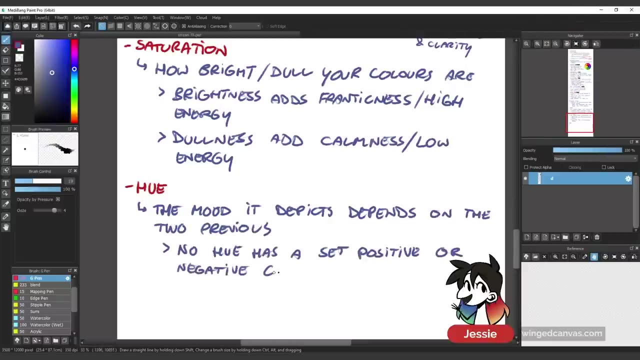 you could use those blues for sadness, Maybe you could use it for melancholy, All that fun jazz. But it depends on how you mix the two of them. And then, last but not least, you have your hue. The mood that your hues will depict will depend on the two previous. 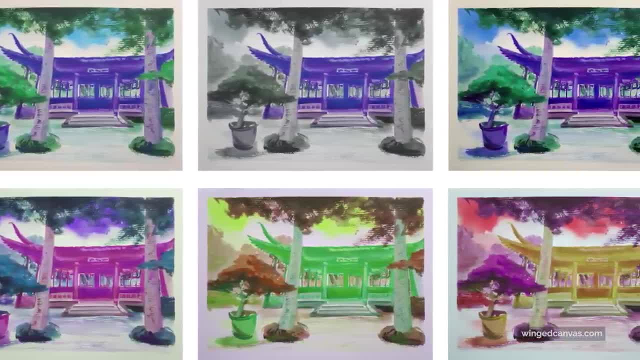 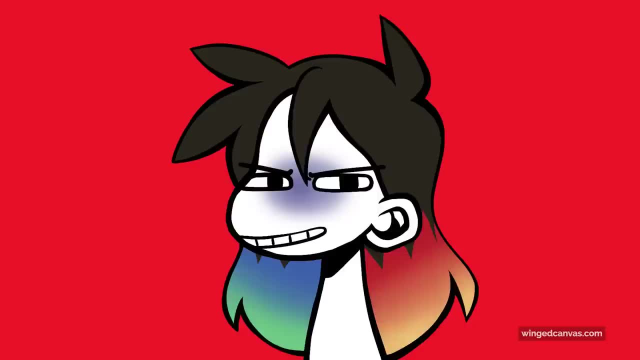 They will depend on saturation and value. How bright or dull and how light and dark that color is will determine the mood You can use red. Red is a color that everyone's like. oh, it's the color of love, or anger, or passion. 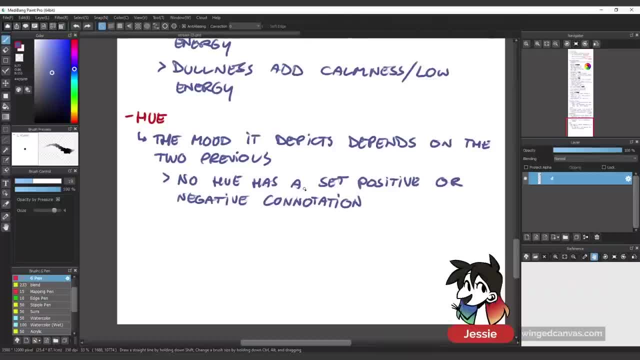 Technically the truth, But you can use it in a lot of different ways. A very bright, somewhat high saturation, high value kind of red. right It becomes a little bit more pink. In that case it could be more childish but it could be more panic inducing, depending. 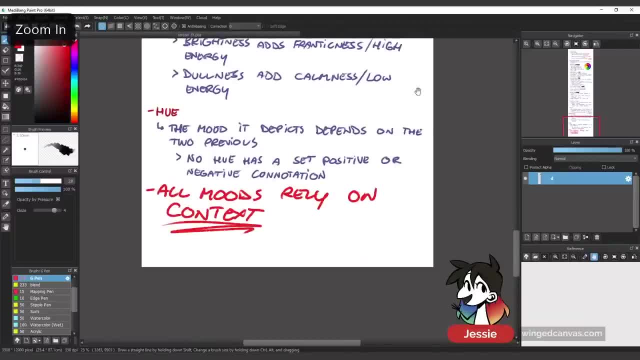 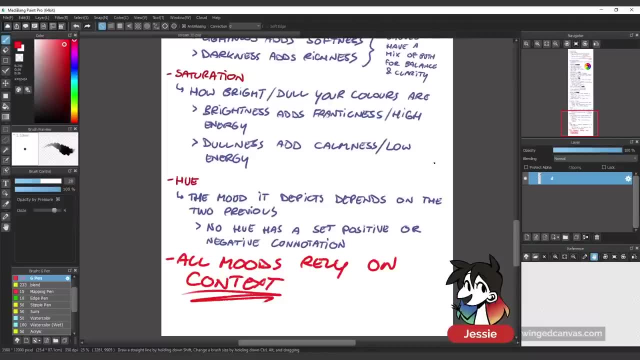 on how you choose to use it. depending on the context. Everything here can be thrown out the window with the right context. At the end of the day, it's the context that you're using. the colors will matter the most with your colors. So without the context, your colors don't matter. You need 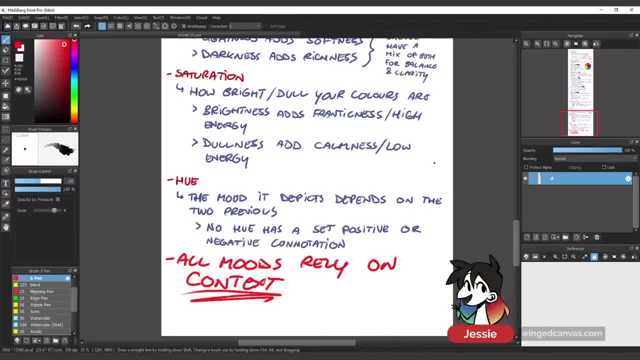 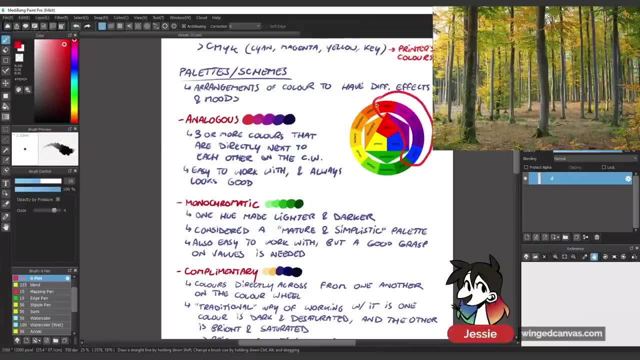 that context in there in order to portray those moods. Same thing goes with backgrounds, though. If I have a forest, I'm probably not going to be using a lot of this side of the color wheel, because these colors are not what you think of when you think of a forest. You think more on. 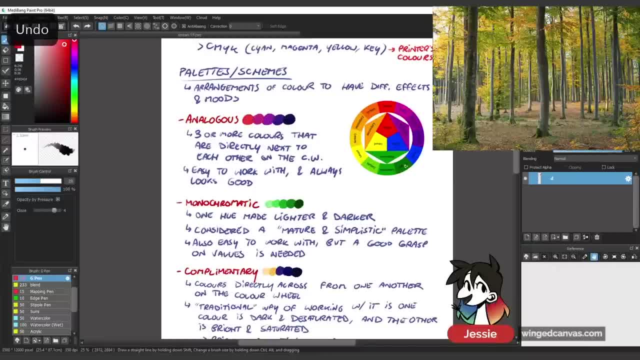 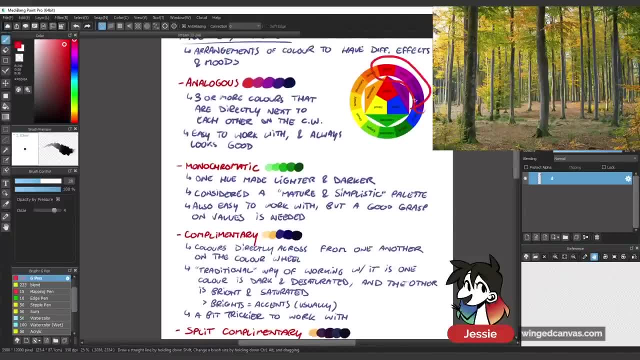 this side of the color wheel, Your oranges, which can be turned into browns, your yellows, your greens- right, Those feel a little bit more foresty, Maybe a bit of blue if you want some water in there. Even then, you probably won't see a lot of purple and red, because that doesn't. 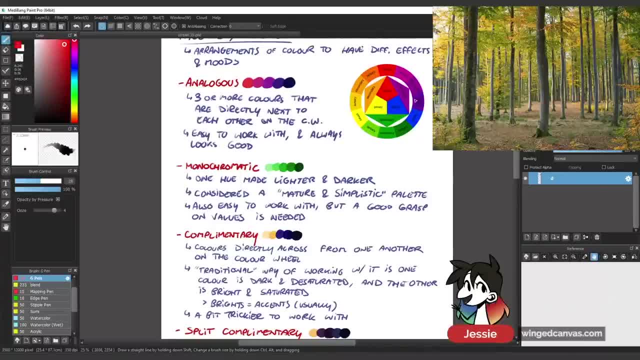 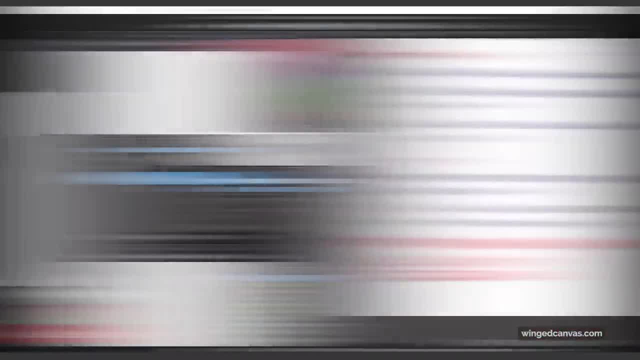 really make sense in the case of a forest. But if you have a forest, you're going to see a lot of of a more reality, more grounded kind of looking forest. So all moods, all colors rely on context in order to work. I'm going to be creating a composition that gives off the mood of fear. 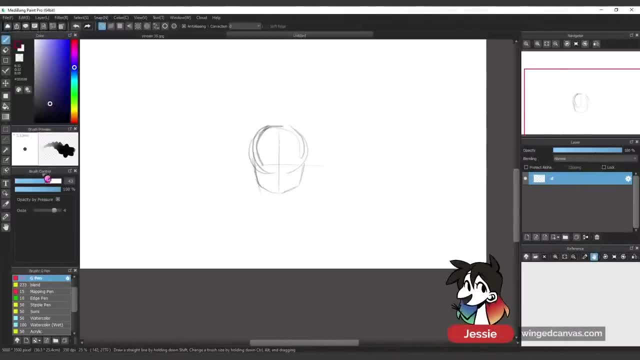 Not necessarily to scare you, but to show a character who is scared, To kind of give off the idea of what a more scared scheme might be with A lot of horror. loves their monochromatic palettes. They love monochromatic stuff, or complementary, Complementary is usually used. 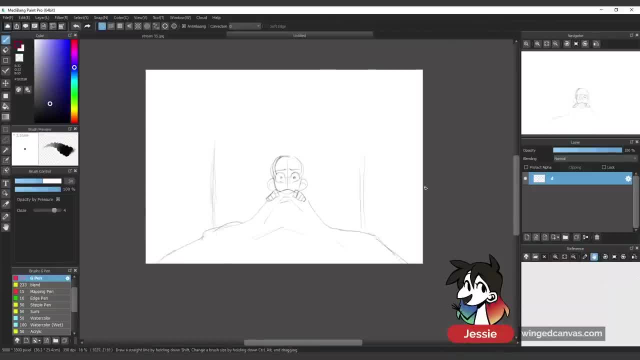 with a lot of space horror, cosmic horror. On the other hand, there's a lot of monochromatic things that they love. On the contrary, a lot more classic horror, even Slasher. they really like monochromes. Older Slasher uses complementary quite a bit, Actually triadic sometimes as well. 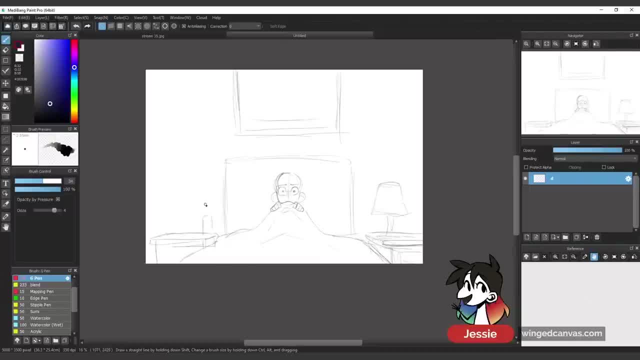 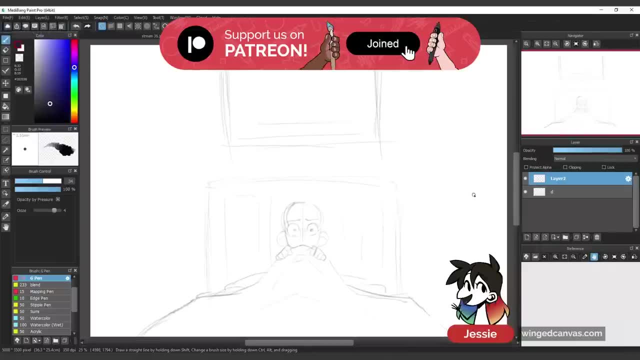 though not often, But more often than not, you'll see a lot of monochromes within dull monochromes within your horror. If you'd like to support the channel and the creation of free arts education, become a member on Patreon. So I want to kind of capture the feeling of late night paranoia. 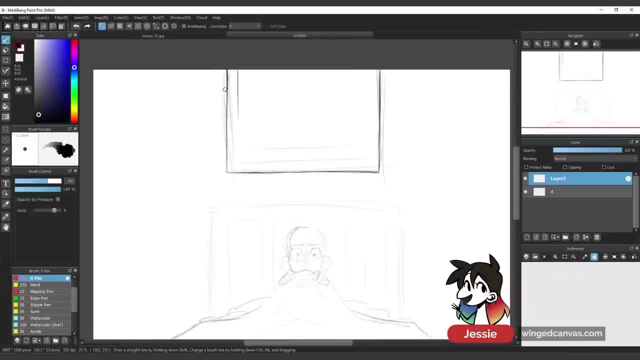 which usually makes you feel like you're really scared of the horror. I don't know if you're necessarily scared of it or not, but I think I have a really strong feeling towards it and it kind of doesn't matter what you're doing with me, so it's not very boring. 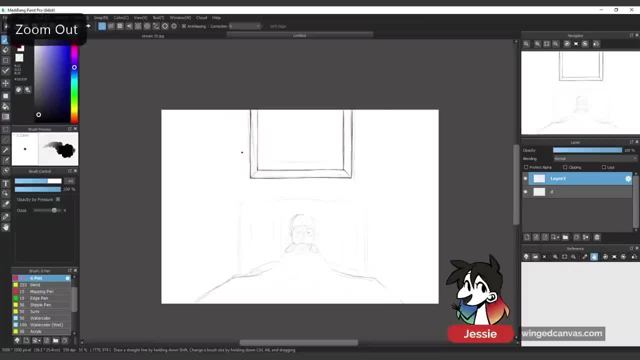 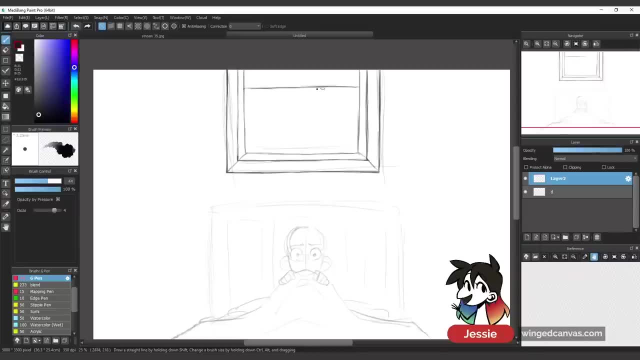 Doom itself, Doom as a feeling. There's two types of ways you can portray Doom right. There's the frantic, somewhat intense emotion of impending Doom and then it's slow kind of realization of Doom, The slow kind of realization. 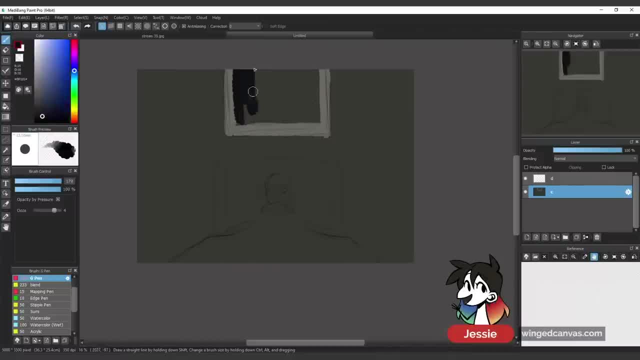 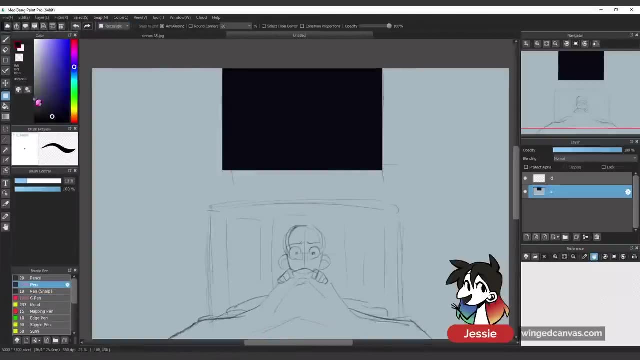 I would stick with with less saturated colours. I'd probably stick with very low, low colours overall, right. that kind of gives you that slow sense of sadness compared to the frantic, like oh my god, the world is ending, i've got to run around everywhere real quick, that one. i'd use very bright frantic colors. 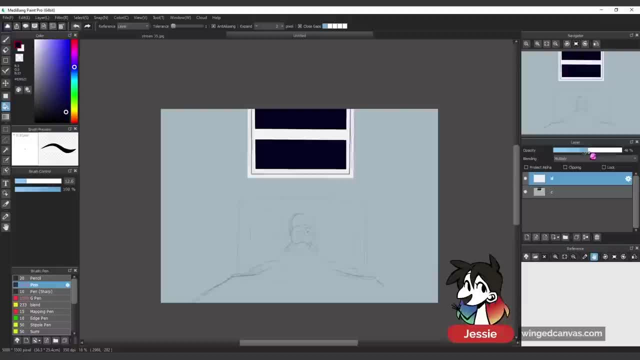 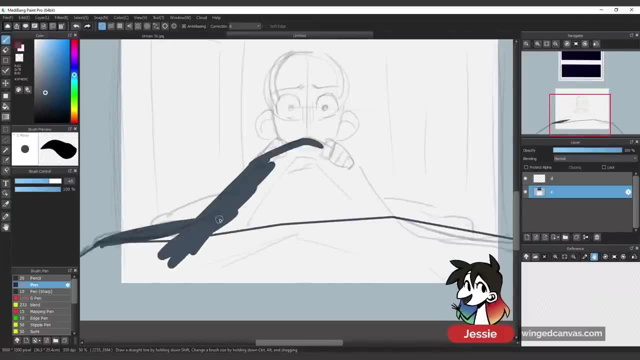 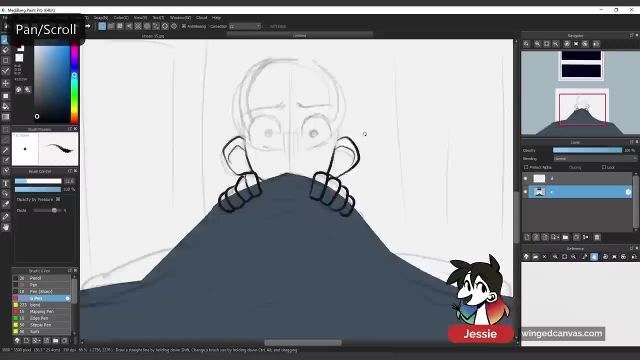 for still kind of dark but a little more frantic, i think much brighter depends on the subject matter of how the doom is occurring. blues and purples: whenever i envision um, blue, purple and black, that's very cosmic to me, very, very cosmic. so that's always how i think of 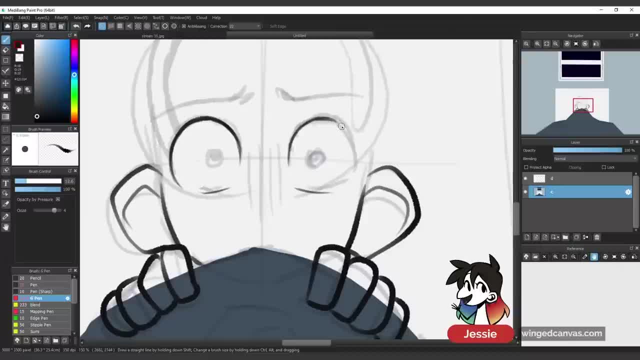 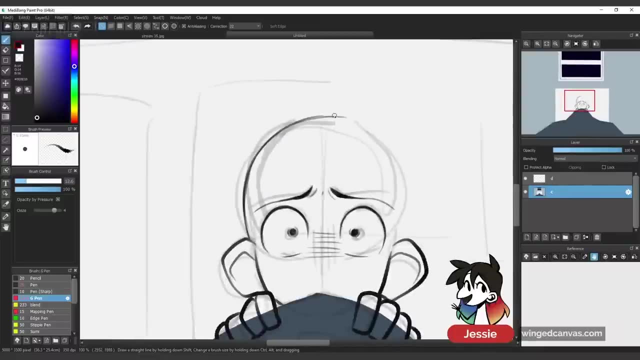 it when i think of doom. it's like i think of impending doom. i would use some blues, but i also might go for some dull yellows and greens. in that case it'd feel more like the same feeling that, um, i don't want to set the world on fire, but the ink spots gives you. i think that's a good. 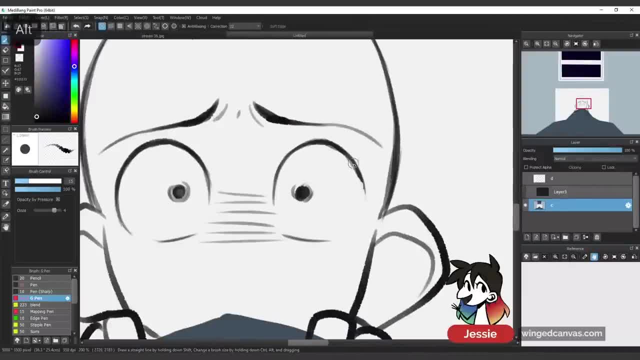 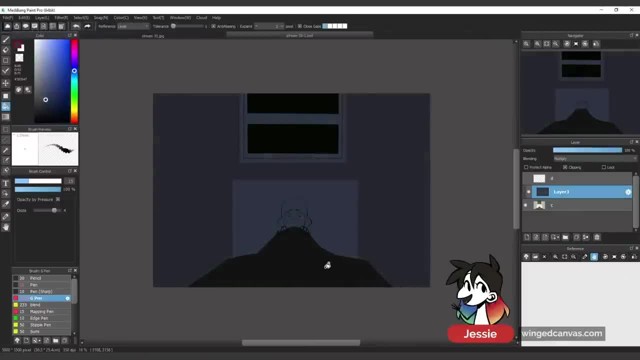 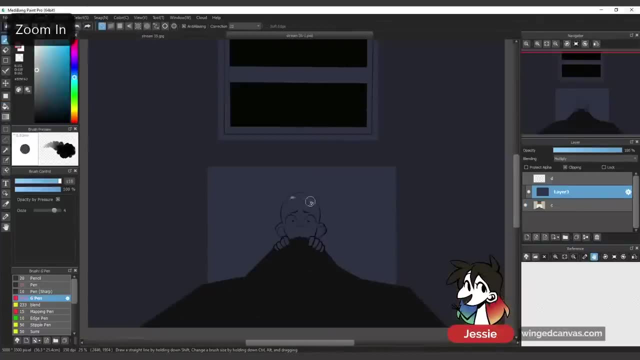 um, a good comparison, or good enough comparison that i can give you. it's like i could go for the blue, which is more realistic, but i feel like it doesn't have the same energy to it. maybe i need to change the color, oops, because i want something warmer. so i'm like 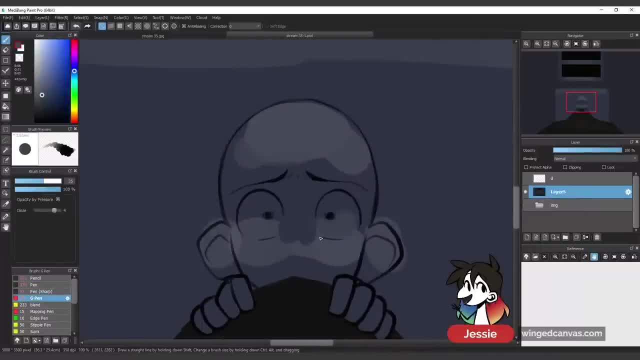 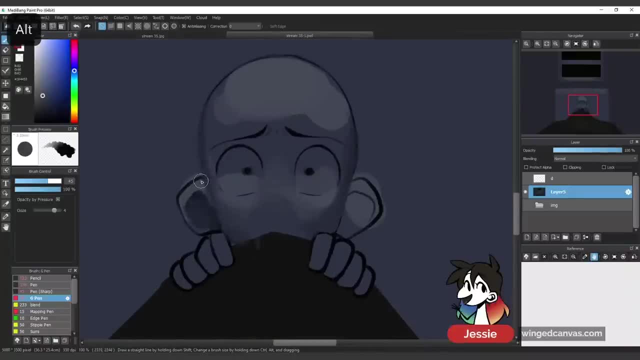 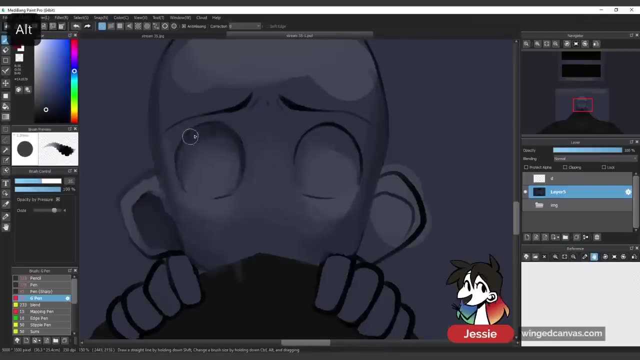 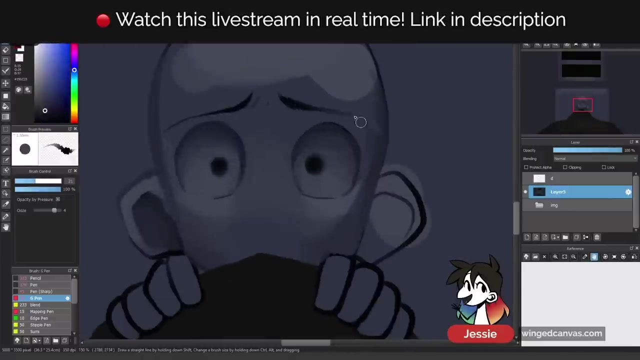 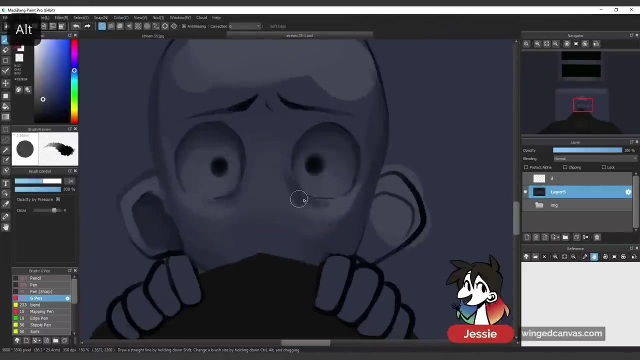 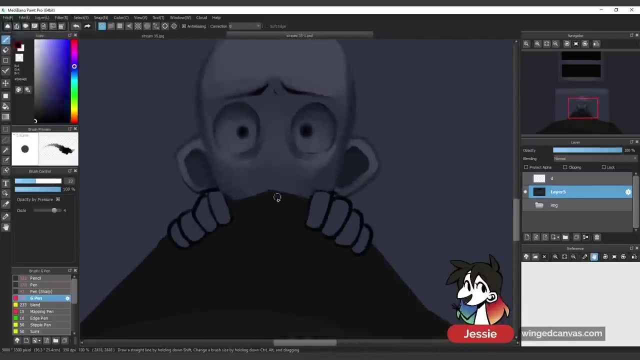 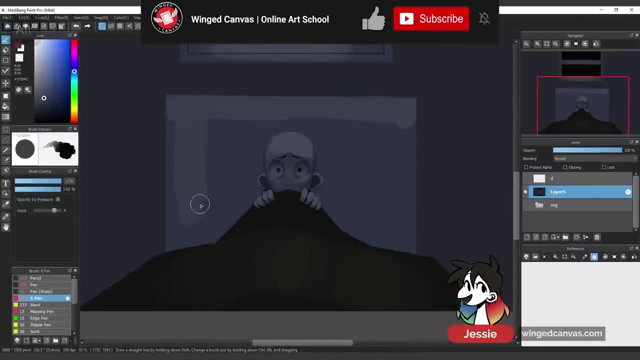 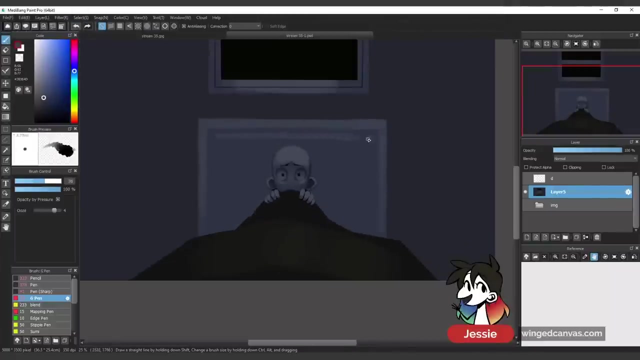 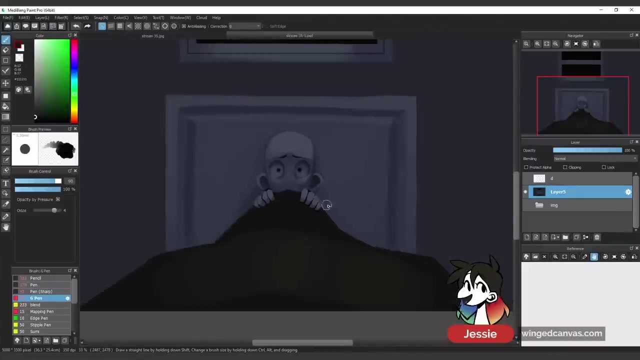 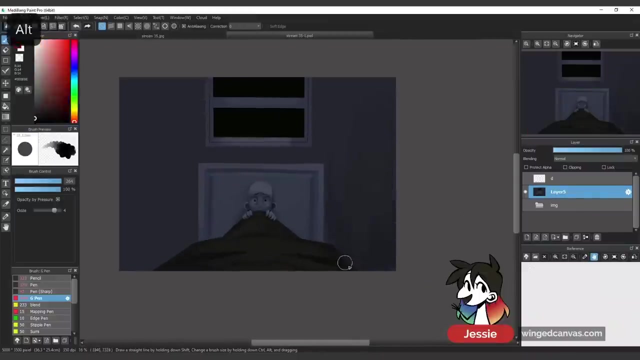 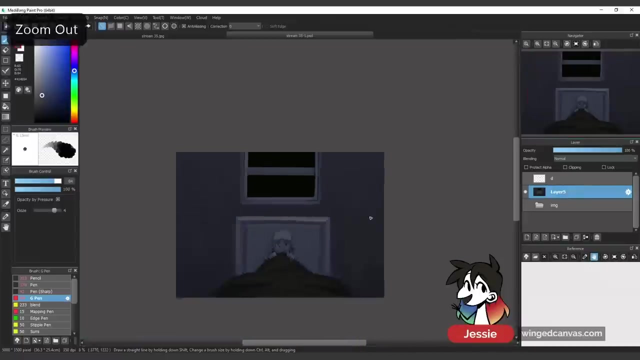 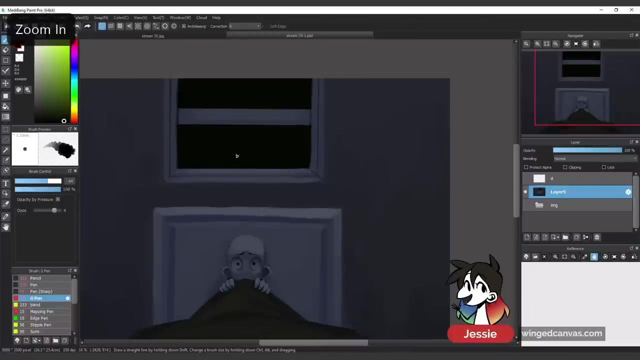 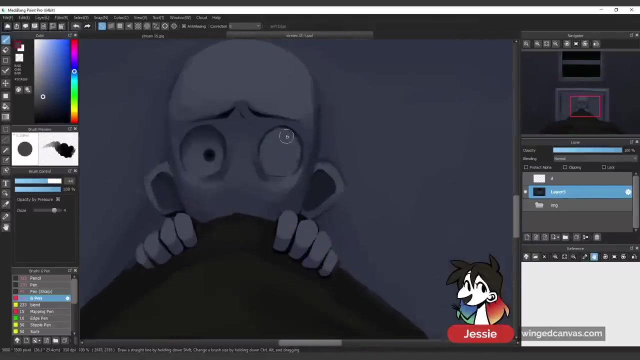 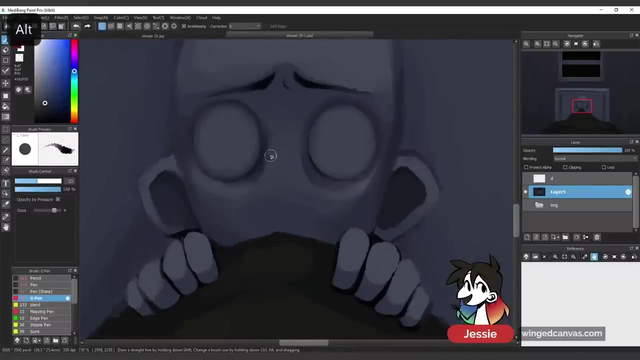 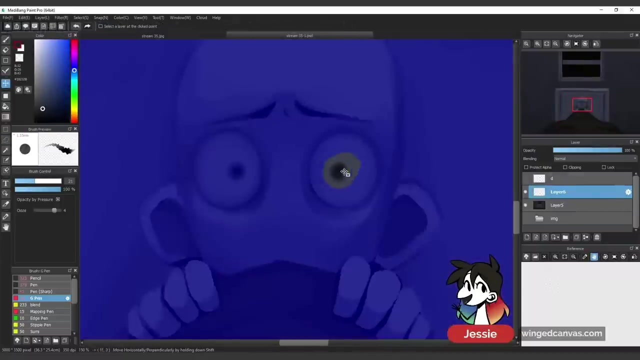 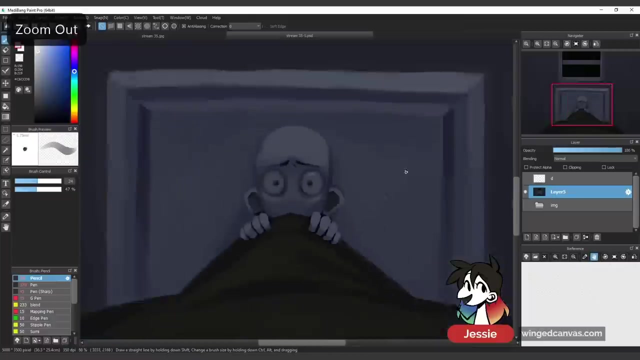 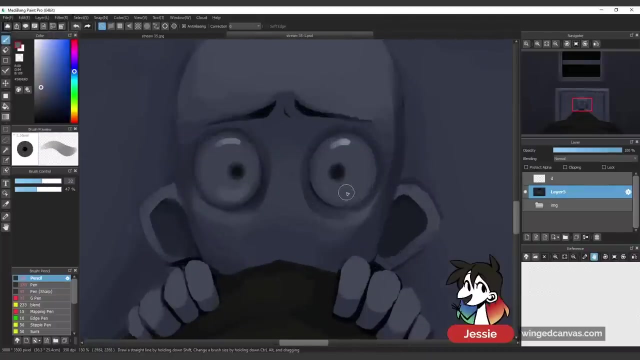 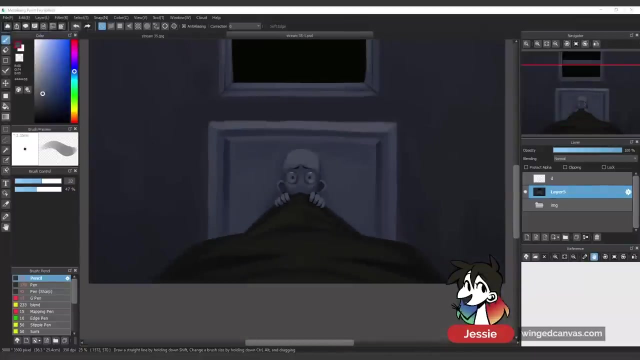 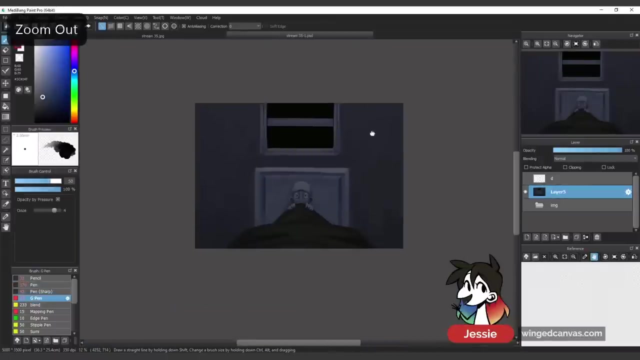 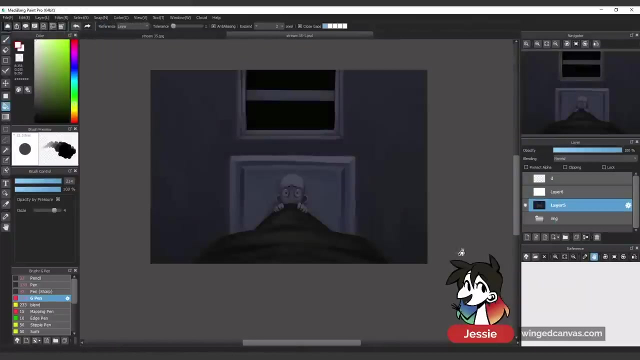 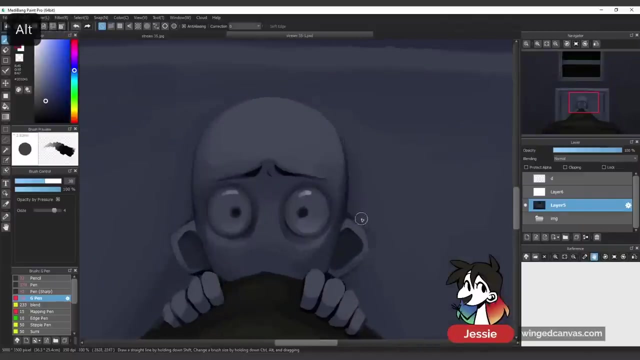 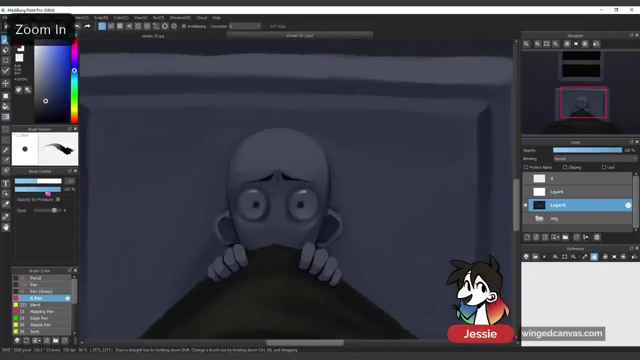 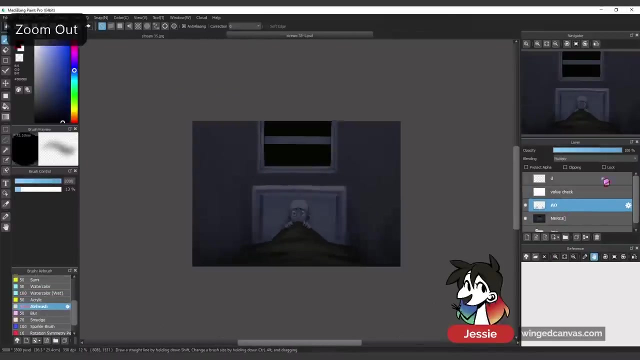 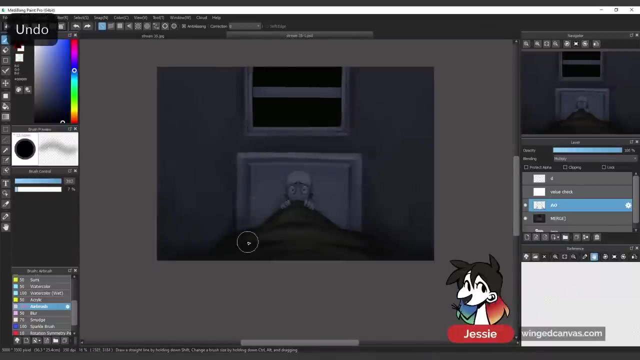 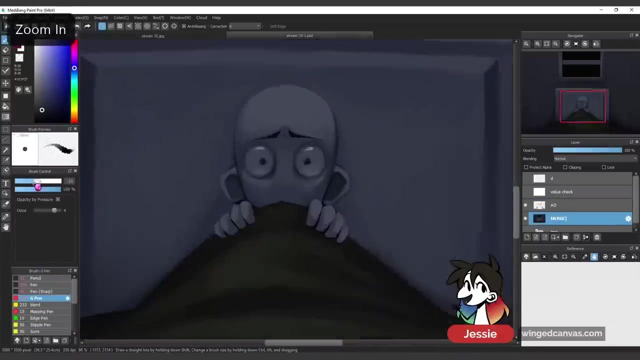